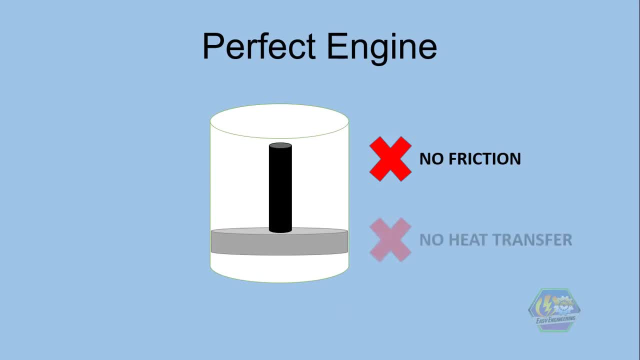 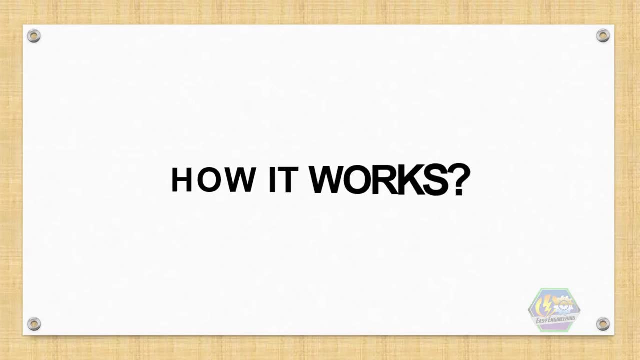 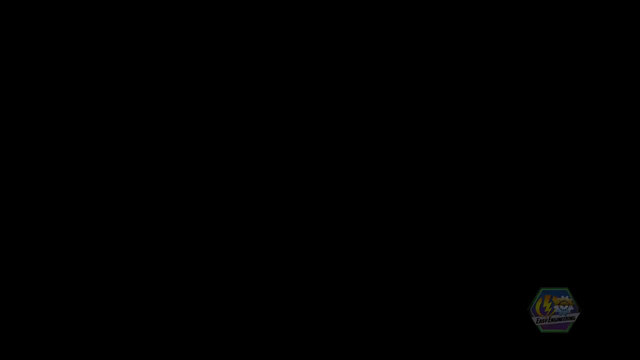 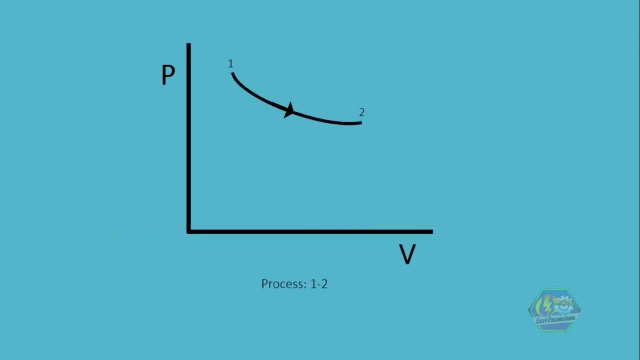 and no heat transfer between piston and surrender balls. Now let's discuss how this interesting cycle works by exploring its processes, the four reversible processes. So now for the first process, process 1 to 2. This process is called isothermal expansion. Isothermal in thermodynamics means no change in temperature, or in other words, 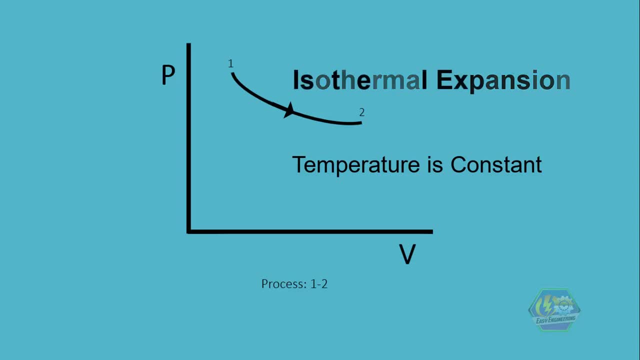 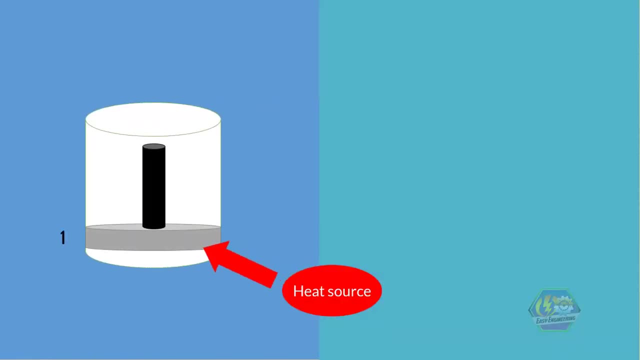 temperature is constant or not changing within this process. So what happens here is that the heat energy from the heat source is transferred into the ideal gas. As a result, the gas expands, which then increases the volume and decreasing the pressure. Now next process 2 to 3, which is called an adiabatic expansion- Adiabatic in thermodynamics. 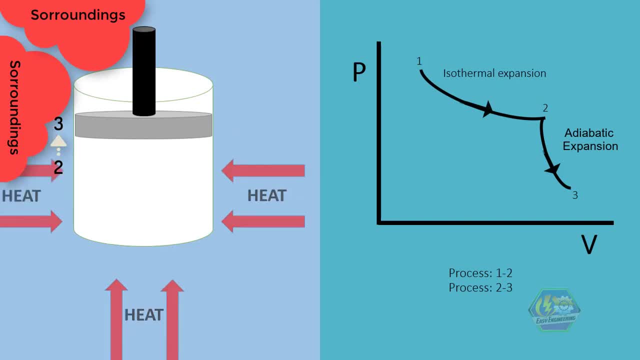 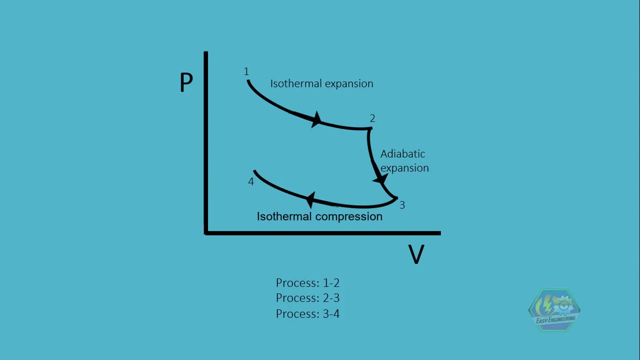 means that there is no heat transfer between surroundings and your system. or, to put simply, all change in temperature is contained within a system which, as a result making the entropy zero On this process, our volume increases and pressure decreases. Third process is the isothermal compression. So by compression it means volume is decreased. 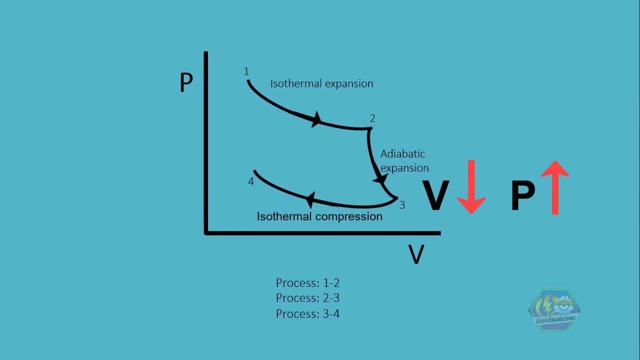 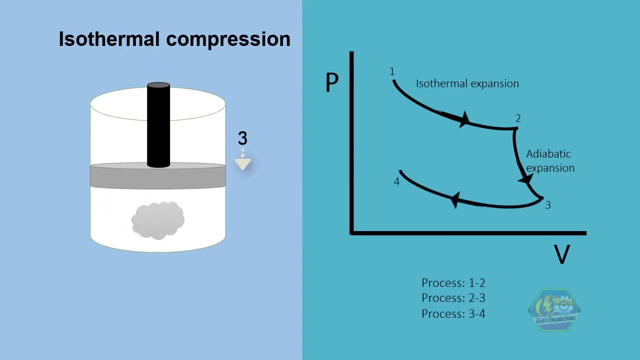 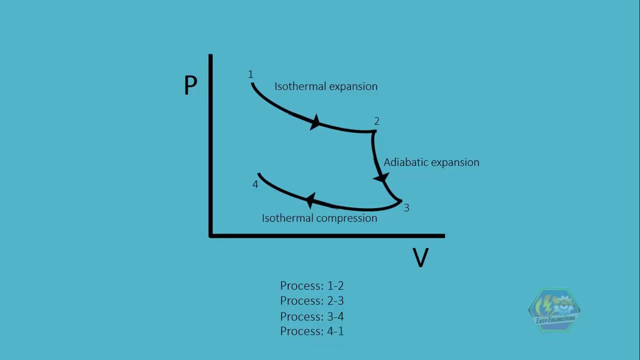 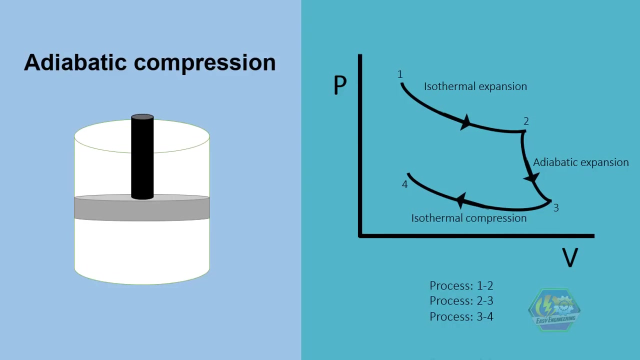 and, as a result, pressure increases. SECOND PROCESS: Clear enough, I think we can pass for a few examples On this process: heat energy from the gas is transferred into the heat sink. And finally, the last process. The last process is called adiabatic compression, Since it's 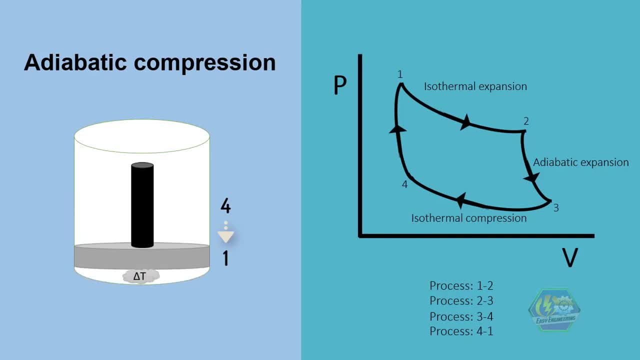 an adiabatic. all change temperature is contained within a system And our entropy really is increasing and everlasting. right, There is no Chrysomy, right, entropy is zero. also, since this is compression, it means our volume decreases while our pressure increases. so that's it. that makes it a cycle. so 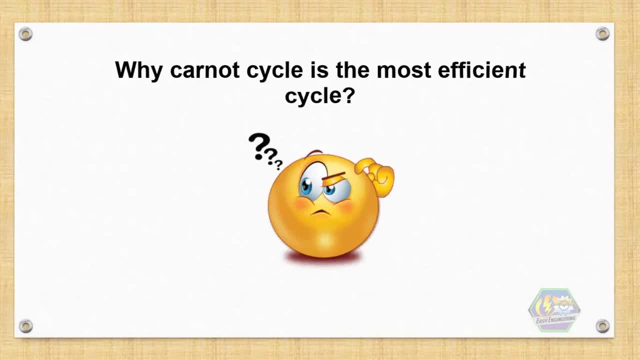 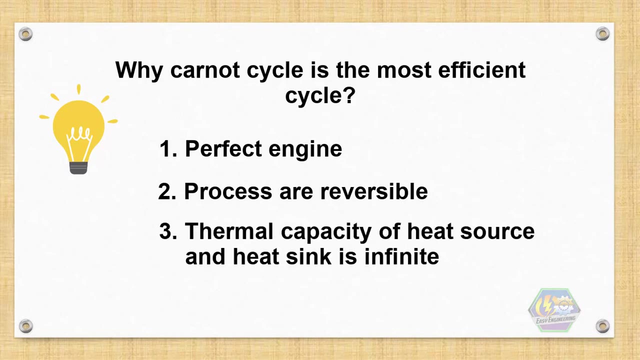 now let me ask you this: why Carnot cycle is the most efficient cycle? well, it's because Carnot cycle is a perfect engine. the process are reversible, working medium is an ideal gas and, of course, the thermal capacity of heat source and heatsink is infinite, which makes no reduction to both during heat transfer.